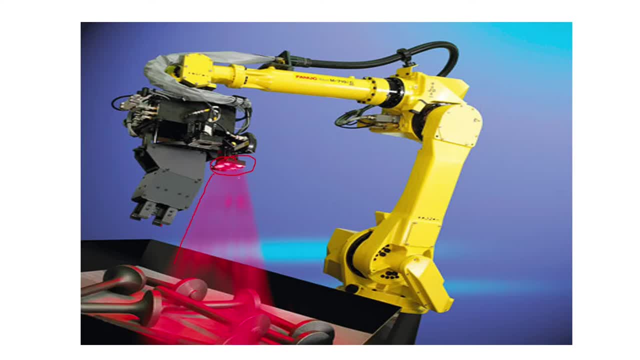 And here you can see, it is going to capture this image here And this image will be a captured and based on its next task. the information taken from this image will be given to the controller of the robot And then the controller will decide what should be the next task. done So, vision is going to help a robot. Okay, so here going with the definition. basic definition: 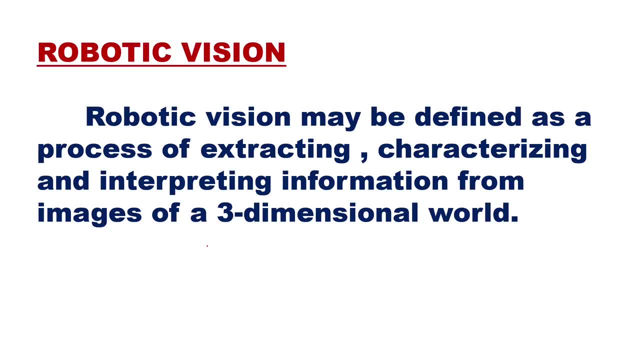 What do we mean by robotic vision? Robotic vision may be defined as the process of extracting, that is, obtaining, characterizing and interpreting. that is, you are going to understand the data and that you are going to interpret it, interpreting information from images of a three-dimensional world. 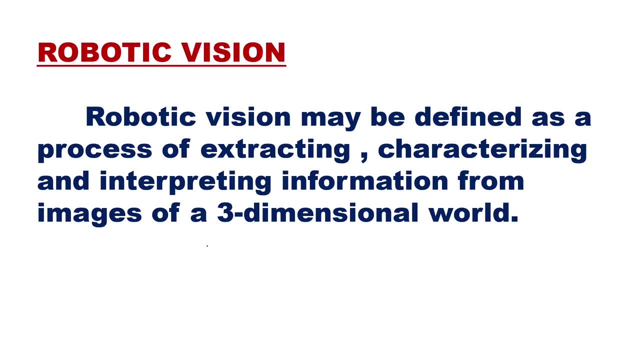 Robotic vision can also be termed as a computer vision or machine vision. It is an important sensor technology with applications in many industrial operations and other things. okay, So there are many applications and it is one of the important sensor technology. Now, here in today's topic, we are going to see the functions of robotic vision system. 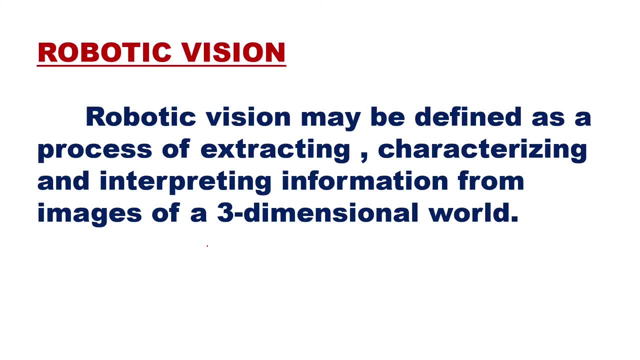 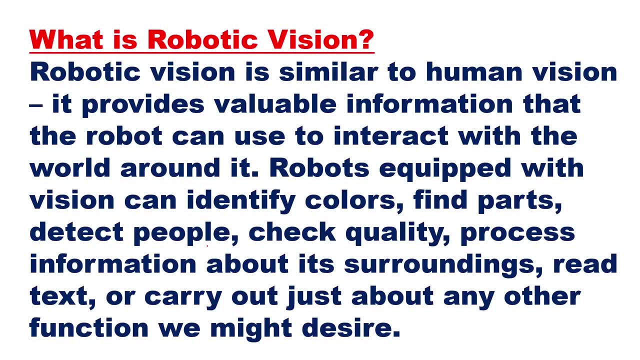 and components of robotic vision system. What are the different units used in robotic vision system, So what exactly it does? So first we will see elaborately what is robotic vision. again, Robotic vision is similar to human vision, as I have told you earlier also. 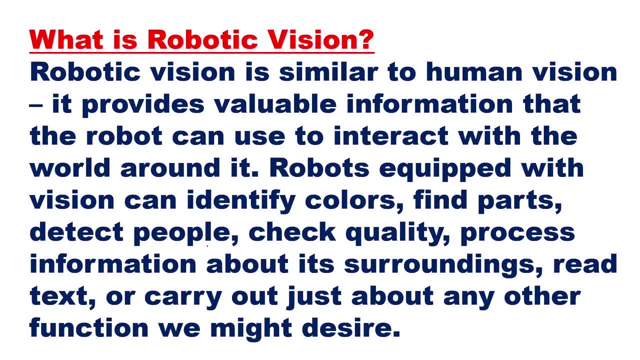 It provides valuable information that the robot can use to interact with the world around it. Robots equipped with vision- that means robots which have vision- can identify colors, they can find parts, they can detect people, they can check quality, they can give information. 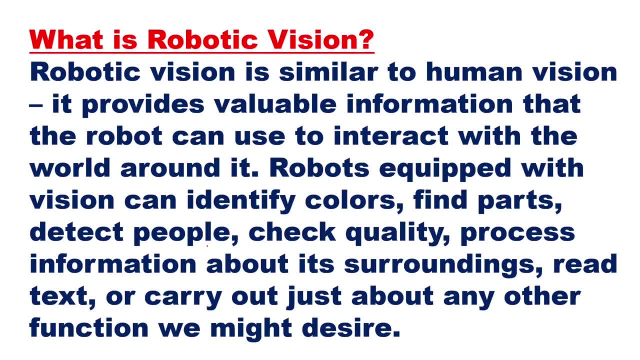 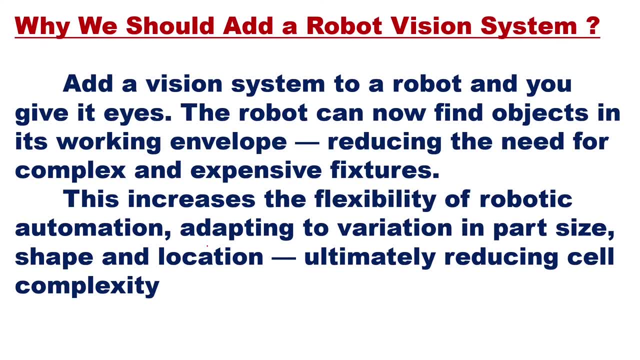 to process information about the surroundings. they can read text or carry out just about any other function we might desire. Then why we should add a robot vision system? Why there should be a vision system for a robot? Okay, anyhow, it is going to work on our commands only. 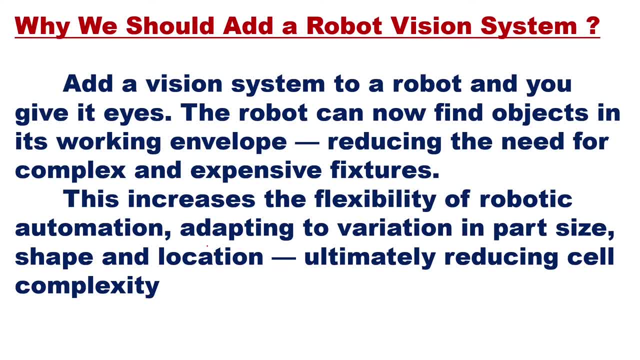 Then why a vision is required. How does a vision is going to help? Okay, so here, add a vision system to a robot and it will give it the eyes. So once you add the eyes, it will give it the eyes. So once you add the eyes, it will give it the eyes. 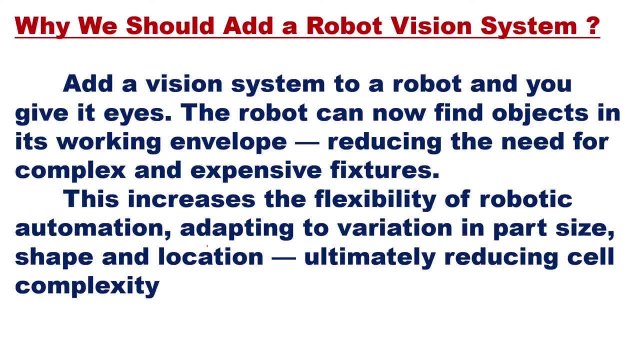 So once you add the eyes, it will give it the eyes. The robot uses appropriate cameras to the robot. It is going to give the eyes to the robot as we have in human beings. The robot can now find objects in its working environment. 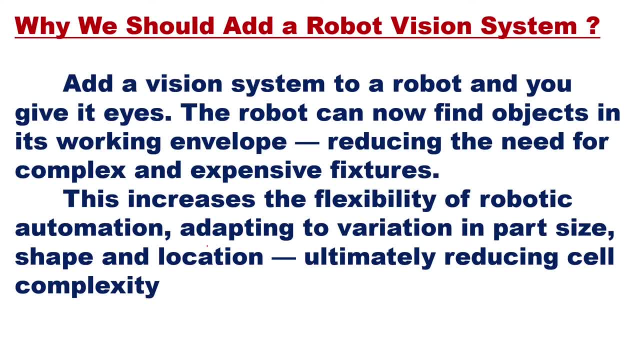 So in its working environment, in its surroundings, the robot can now find objects by just viewing it, reducing the need for complex and expensive fixtures. So it doesn't have to go and touch things and then understand what it is okay, It can just view and then can understand. 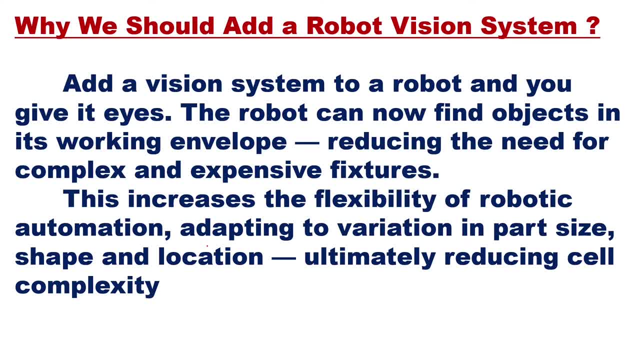 understand that there is some object, okay, and that can give the information. now, this facility, this increases the flexibility of robotic automation, adapting to variation in part, size, shape and location. so ultimately, many things will differ because of the vision, ultimately reducing cell complexity. so here we have seen now basic definition of robot vision system and we have 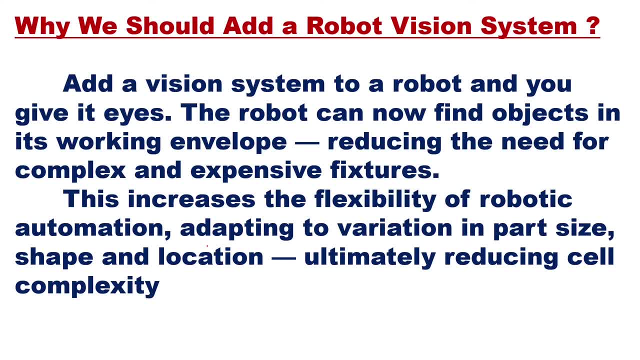 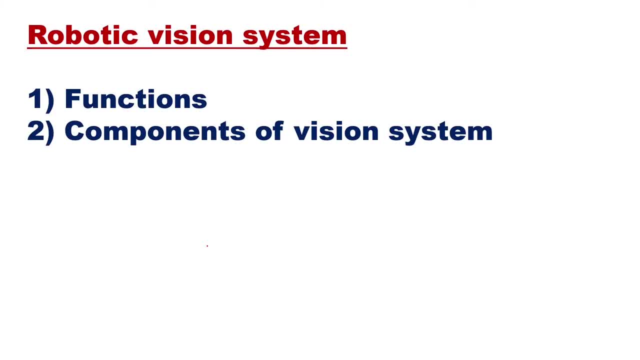 also seen why we should add a robot vision system. okay, why a vision system should be added to a robot. now. then we will go to see the what topic, that is, robotic vision system, and in that we are going to study two things. one is the functions of the robotic region system. what are the functions? 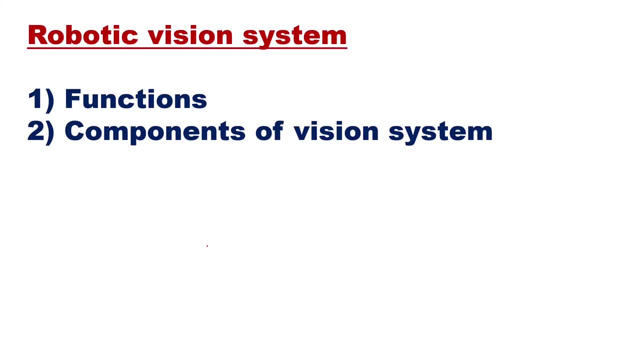 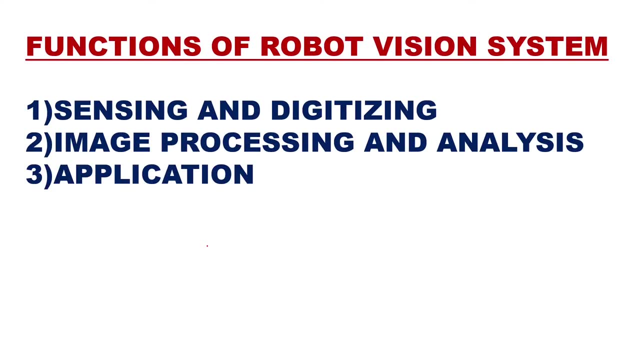 and then what are the components or the units of the robotic region system. so first we will see the functions now in this functions of robot region system. number one is sensing and digitizing, number two is image processing and analysis and number three is application. okay, now what are these sensing and digitizing? what is image processing and analysis? 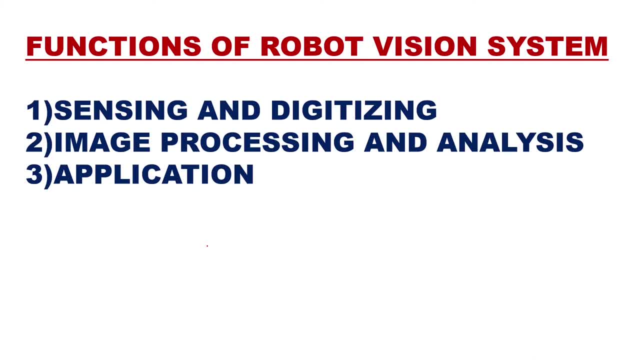 what is application? so, as we know, the front end of the camera will be having the option of sensing things. okay, so it is going to take the image, it is going to capture the image, then. then the image will start to move, but when we look it will begin to move. i mean, it will begin to move. 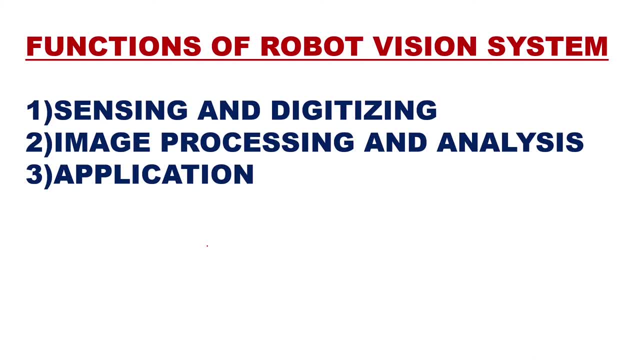 image, which is analog, will be converted into digital and after converting into digital, it will be processed where it can be reduced in noise, enhanced in data. okay, image will be enhanced and the data, each particular data of that image will be taken, analyzed, given to the controller and then 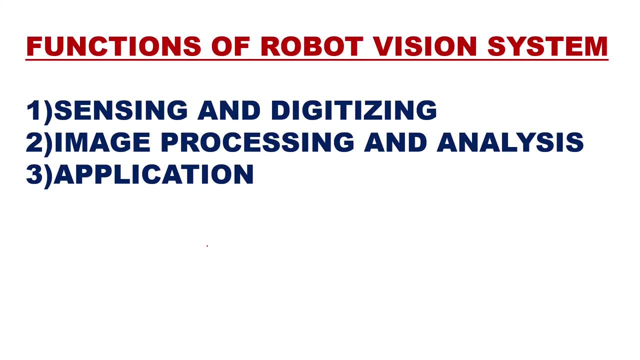 the controller will give a command to the manipulator and the manipulator will give the particular application. this is how the general flow of the task goes. okay, so these are the prominent things, prominent factors of functions. these are the functions of your robot vision system. so first is sensing and digitizing, second is image processing and analysis and third is 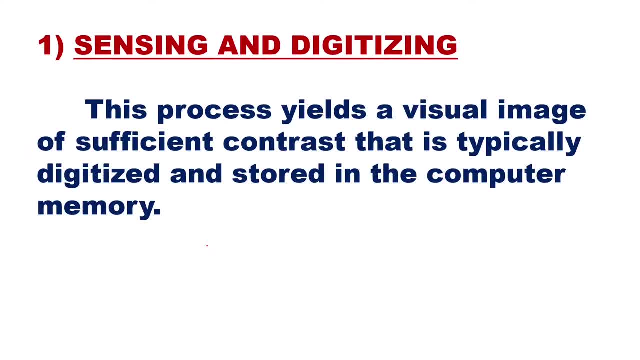 application. so we will see what is sensing and digitizing is so here. sensing and digitizing this process yields a visual image of sufficient contrast that is typically digitized and stored in the computer memory. so sensing means your a camera is going to capture the image. it is going to sense the light reflected. 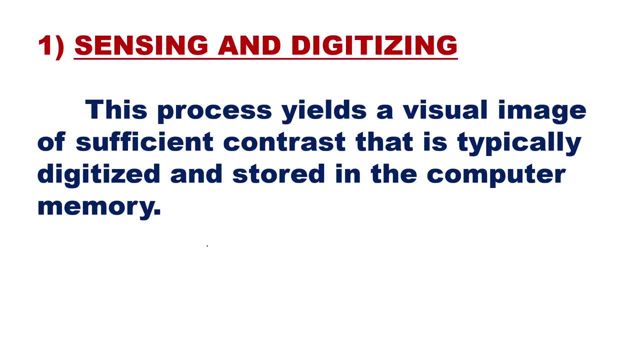 from the image, it is going to sense it, it is going to capture it and then, with a particular transducer, it is going to convert it into analog signal and then, with the help of analog to digital converter, it is going to digitize it and then stored in the computer memory. this is the first function of your robot vision system. 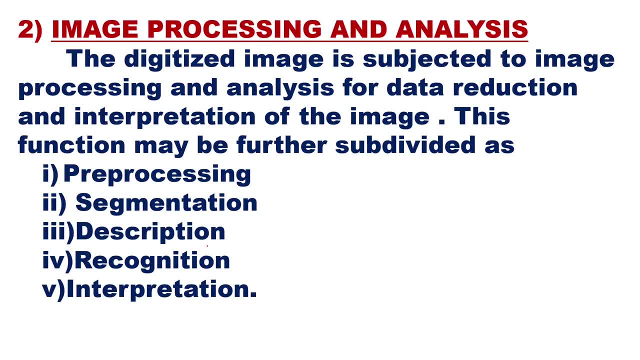 then the second function is image processing and analysis. now what happens in this image processing analysis? the digitized image which is there in the memory is subjected to image processing. that means it is going through a process of image processing and analysis for data reduction and interpretation of the image. 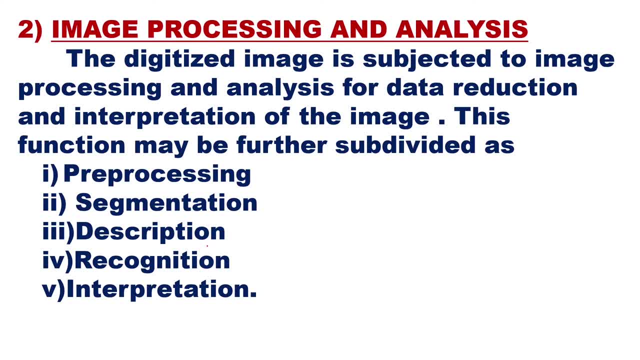 now, if you want to understand the data which is there in that image, then you have to go with the process that is image processing, and then you have to do the analysis. okay, this function, that is, image processing and analysis, may be further subdivided: pre-processing, segmentation, description, recognition and interpretation. now these all. 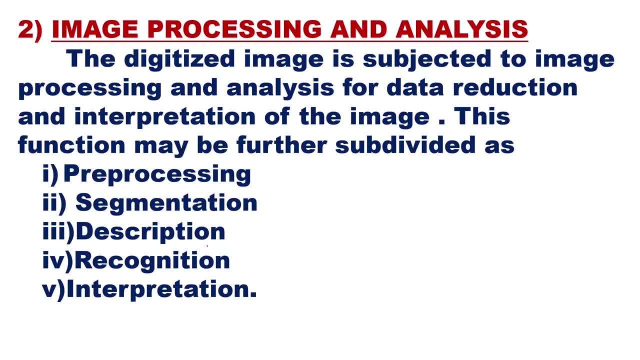 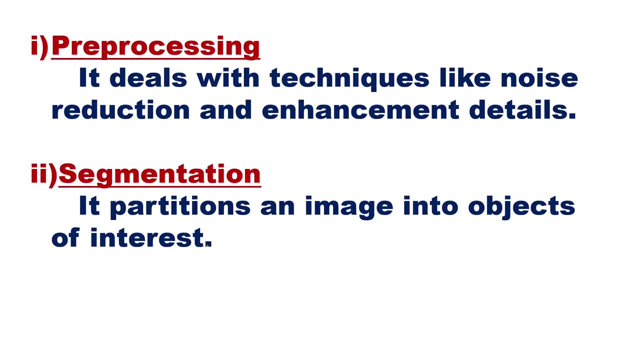 terms are related to image processing. okay, now here, pre-processing deals with the technical processing while selecting other images. so one of our cases we see here: in math, we have prepared the edged image. this time we are going to show how those dataigoed, all our data, to like. 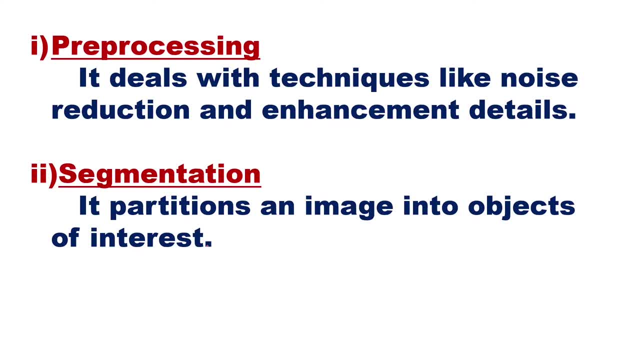 to select or ask what needs to be e-planed to create an image. now the image processing method is similar to what we know from interventional logic. we can see that as all data that is ironically collected are large orders, then it is a double main part. 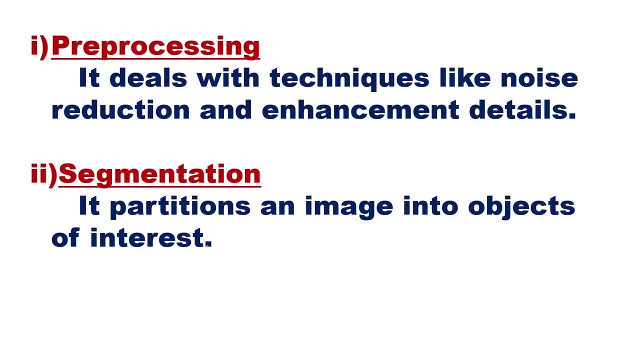 of theFirestone, but even question: you are entitled to the zero slope curve for some kind of time, and so that is what we are coming at, so that then, in this second one, you want to document which one that is looking like gal qua j, quem i am sending you now, means the. 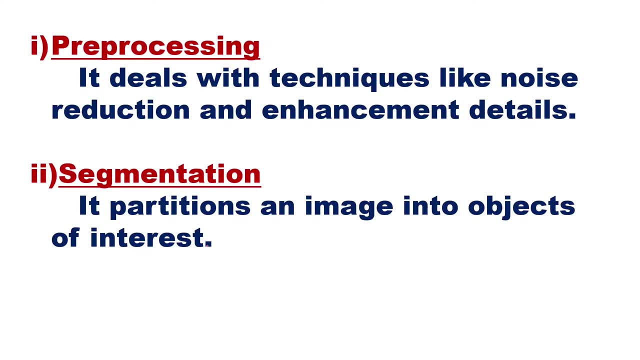 now segmentation. it partitions an image into objects of interest. so it is going to give the parts of the image into objects of interest, means wherever we have a interest in our data. whatever data is important, okay, that important though, that image will be made into partitions so that we can have particular data of our concern. we can study that. so that is called. 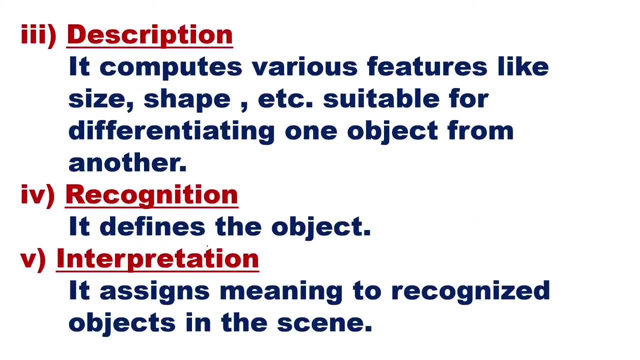 as segmentation, where you are going to do the partitions of the image. then a third one is description: it computes various features like size, shape, etc. suitable for differentiating one object from another. then fourth is recognition in image processing, which defines the object, whatever you have taken image of. then fifth is interpretation: it assigns meaning to the 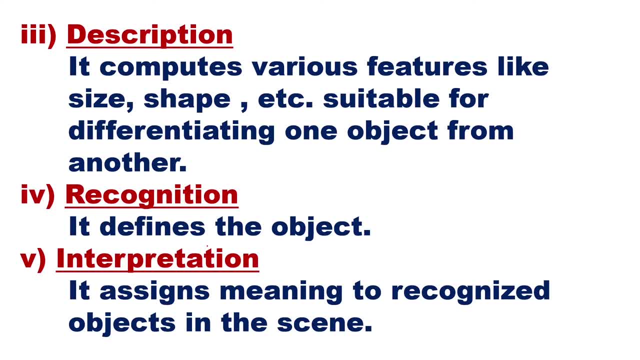 recognized object in the scene. so whatever object, that is, whatever image you have taken of the object, from that, what data you are going to get that meaning? okay, so interpretation process gives it, assigns meaning to the recognized object in the scene. that is the picture, that is the. 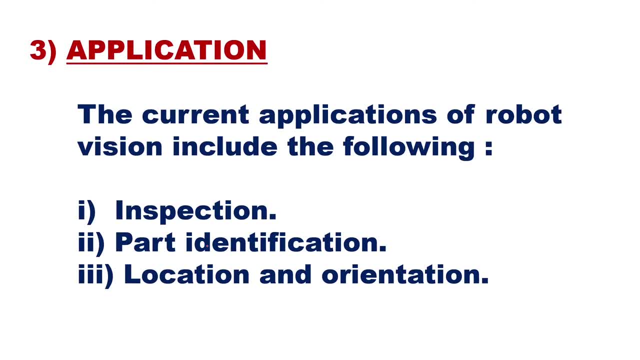 image. then the third main function will be application. the current application of robot vision include the following: it can do inspection, it can do part identification, it can give you the location and orientation of the object. so these are the areas in which we can have application of robot vision system. 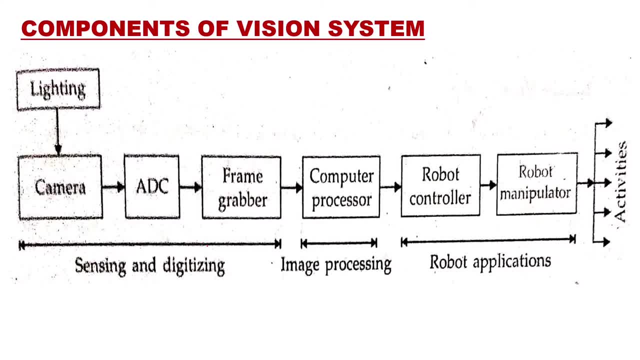 then we will go to see a components of vision system. so here we have shown a block diagram where the first block is shown as lighting here. so the first block here is the lighting. so here you can see, the first block is lighting. now this is nothing but a light which is put on the image of the object that is reflected back. 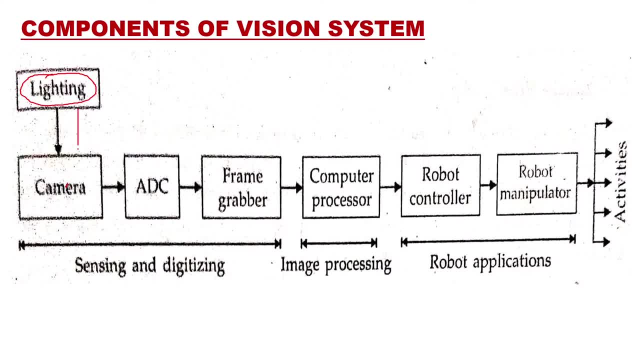 so the reflected light is captured by the camera, the reflected light from the object. so here you can have your object, or whatever vision you're going to have of what part you're going to have or which person you're going to have. what is the picture you are going to have? 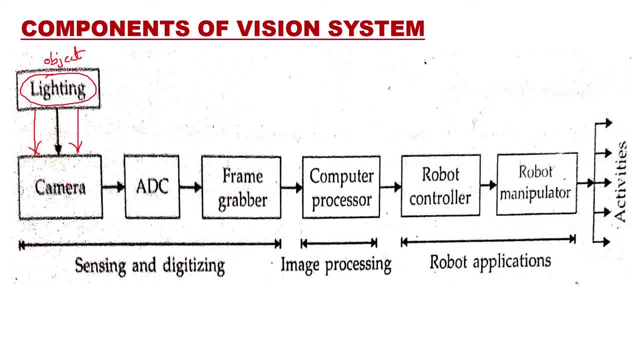 from that picture, the illuminated light which gets reflected back from the object. that reflected light will be captured by the camera. okay, Okay now this reflected light which is captured by the camera will be converted into analog signal by a transducer. Now that analog signal will be there in the camera and that will be converted to digital. 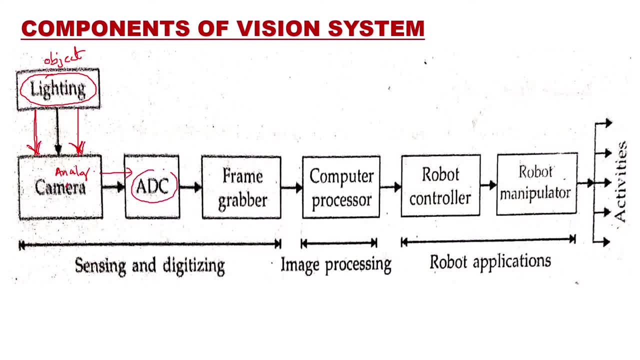 signal by a analog to digital converter. okay, And then after that you have a frame grabber which is going to store the image. Frame grabber is going to store the image. Now, these functions are called as sensing and digitizing. That means you have sensed the picture, you have sensed the image, you have taken the 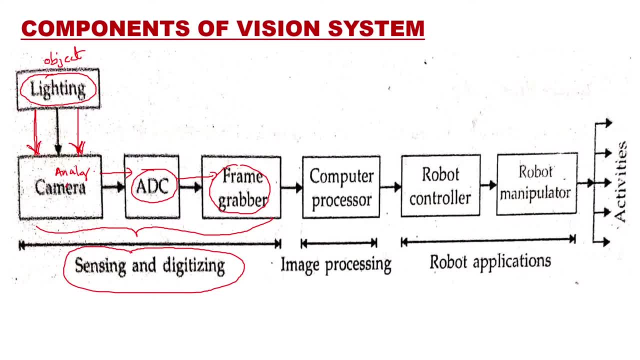 image. you have captured the image by the camera. The camera is going to convert that image into electrical analog signal by a transducer, and then you are going to convert that analog signal into digital by a analog to digital converter and then you are going to store it for memory. 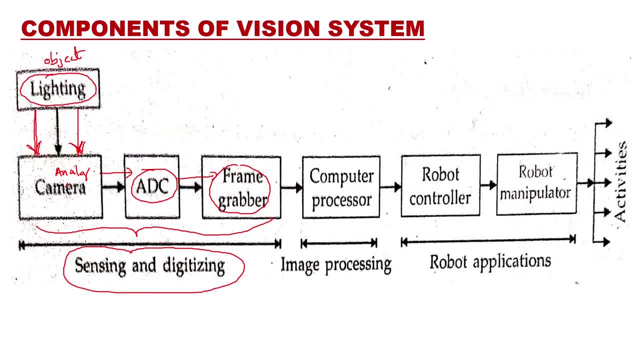 Which is your frame grabber. okay, After that, whatever information you have stored about the picture in the memory in a digitized format, that will be processed and there will be an image processing case. So here you can see, you are having image processing. 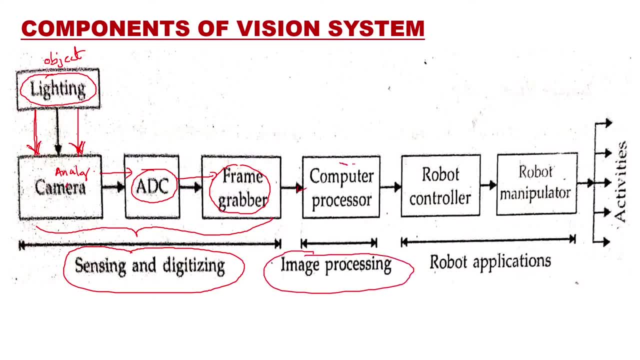 So that will give you the unit of computer processing. So, as we have seen here, here you are going to reduce the noise. So here you can reduce the noise, Reduce noise, that is noise reduction. You can enhance the image, Enhance the image. 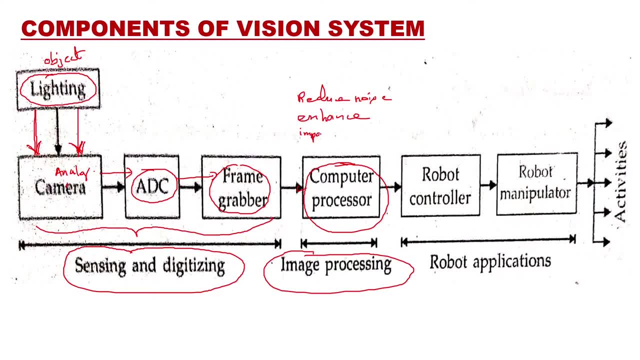 You can concentrate on important details, Important details, that is, important data, okay. And then you can give all that important data to the robot controller, whatever has been viewed by the vision system. Then the robot controller will use its data system and use these inputs and then manipulate. 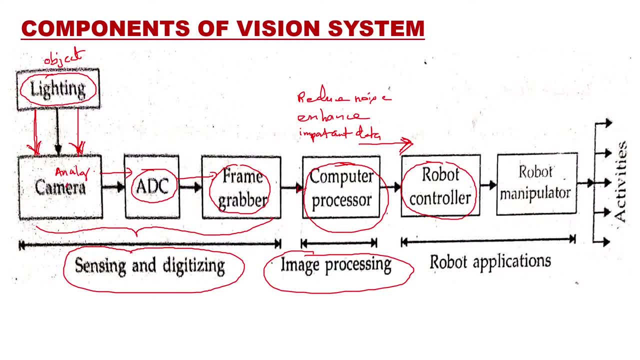 what type of task it has to do further, and then it gives a command to the robot manipulator. This robot manipulator will ultimately perform the particular task and that task will be done. That will come under your robot applications. okay, So the components of vision system is divided into three parts. mainly, as we have seen, the 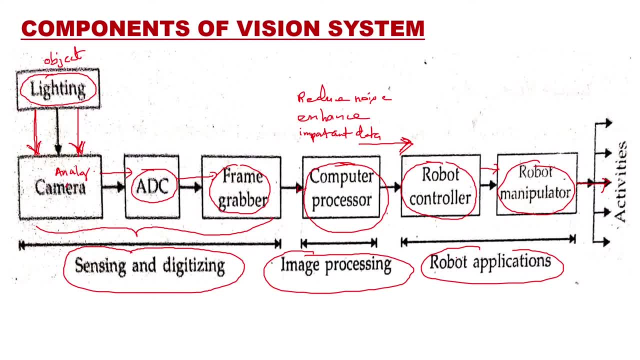 below Names: sensing and digitizing, image processing robot and machine. Okay, application. so in sensing and or digitizing you will be having the light reflected from the object. you are going to first have a source which will illuminate light and that light will go. 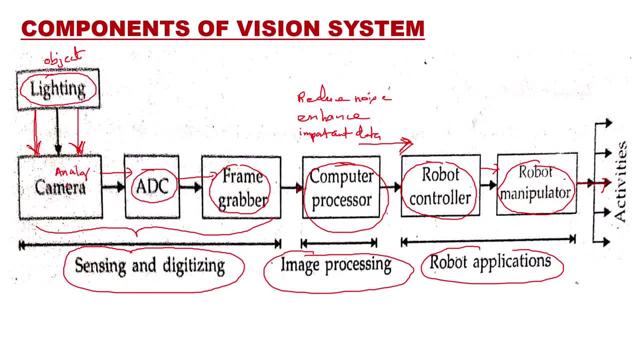 hit the object and it will come back. it will be reflected on the camera. the camera will capture the image and that image, which is in the form of light, will be converted into electrical analog signal by the appropriate transducer, and that analog signal will be converted to digital signal. 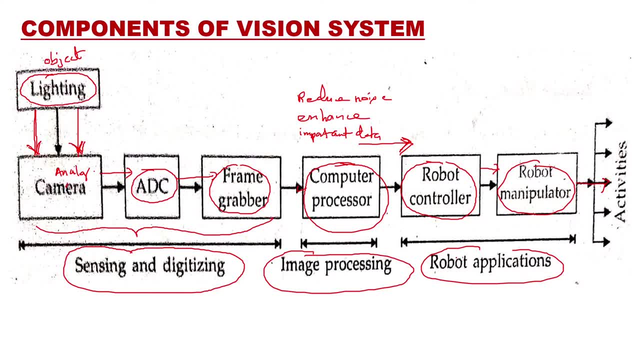 by adc, and then it will be stored in memory, which is called as frame grabber, and then, after that stored, information of the image will be processed in which you are going to reduce the noise, you are going to enhance the important picture details, you are going to enhance the image, you are going 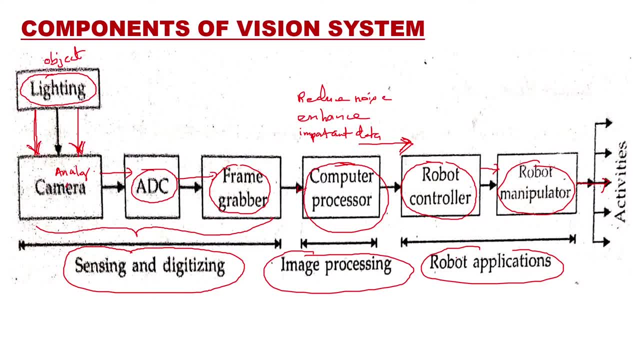 to have the important data. you are going to interpret the important data and that important data will be given, that information will be given to the robot controller, where the robot controller will take that input and, depending on its task assigned, it is going to execute its algorithm and then, according to its software execution, it is going to give a particular 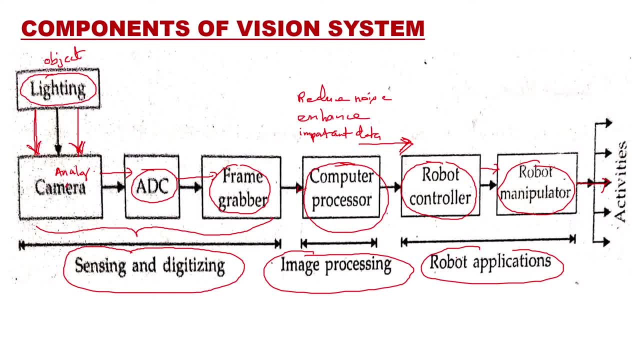 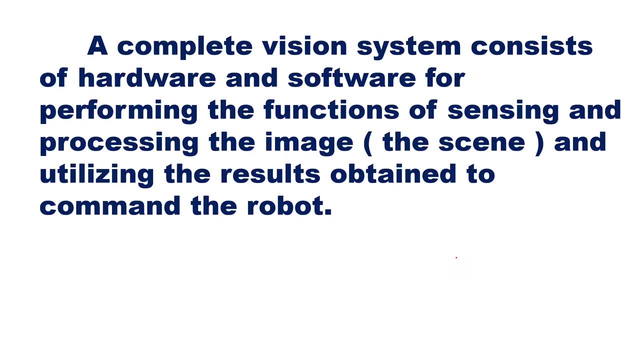 next command to the robot manipulator and the robot manipulator will complete the task. what has to be done next? after the vision, information is given to the robot. so here, a complete vision system consists of hardware and software for performing the functions of sensing and processing the image, that is, the scene, that is a picture, and utilizing the results obtained to. 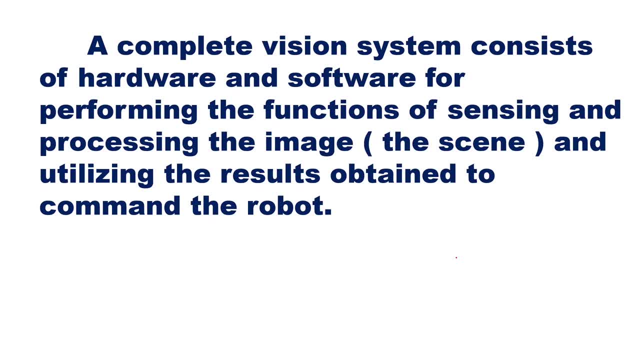 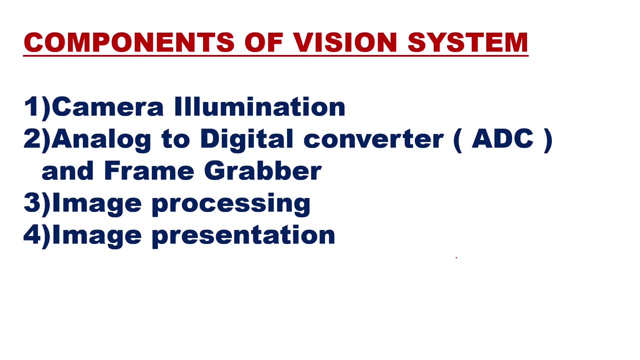 command the robot. so, anyhow, whatever thing you are going to see, whatever the vision system is going to have information, that information will be used to command the robot. then the components of the block diagram, what we have seen now. the first component will be a camera illumination. so in this illumination we will be giving light. 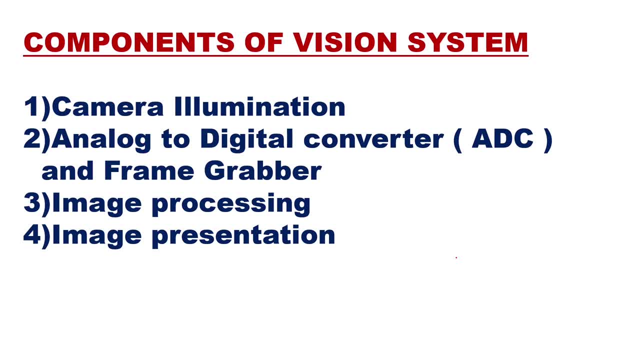 and then the light will be reflected from the object and that reflected light will be taken by the camera. then second one is your analog to digital converter, adc, and third one is the frame grabber, and then you have image processing and then image presentation. so these are the components. 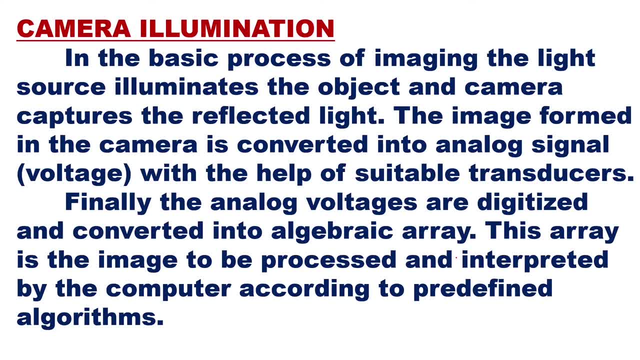 of vision system. then what do we mean by this? a camera illumination, so it is a process of imaging. now, in the basic process of imaging, the light source illuminates the object. okay, so it will provide light which will fall on the object and the camera captures the reflected light. 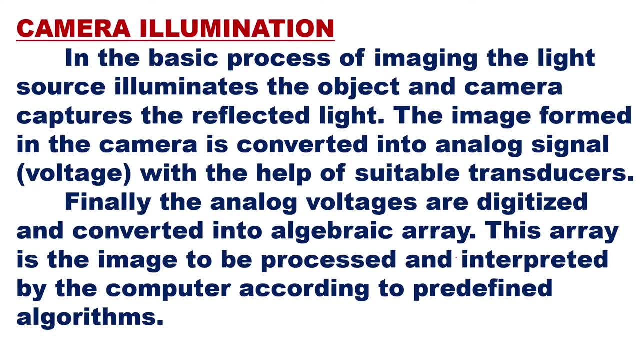 so the illuminator is going to view be a source of light, it is going to put light on the object and the reflected light will be captured by the camera. the image formed in the camera is converted into analog signal, that is, voltage, with the help of suitable transducers. finally, the analog voltages: 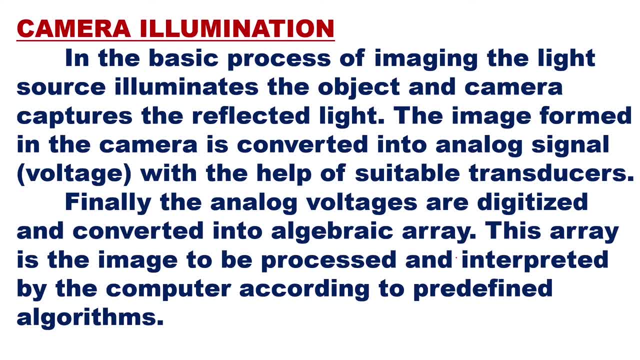 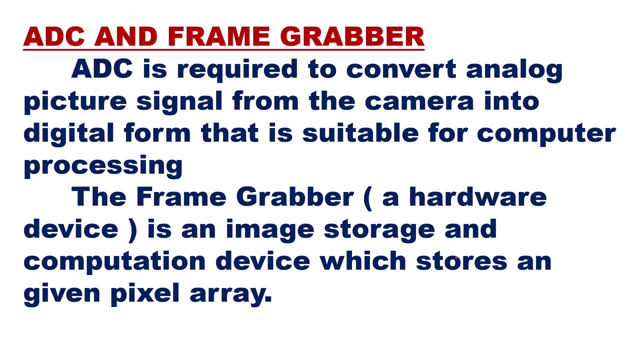 are digitized and converted into algebraic array. this array is the image to be processed and interpreted by the computer according to the predefined algorithms. what are there in the computer then? what is this adc and theありがとうございました? where about, you know, the parallel method and frame grabber, which are the second and the third blocks? 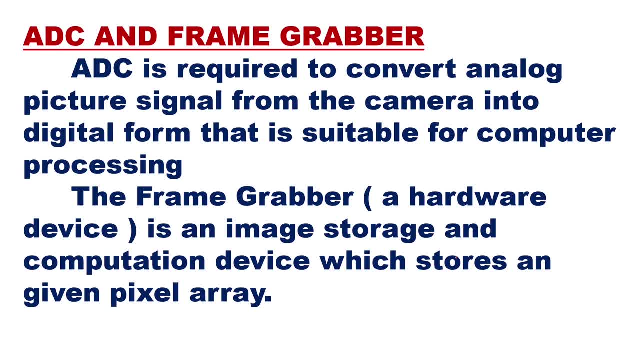 which we have shown in the block diagram. ADC is required to convert analog picture signal from camera into digital form that is suitable for computer processing And frame grabber means it is a hardware device. It is an image storage and computation device which stores a given pixel array. 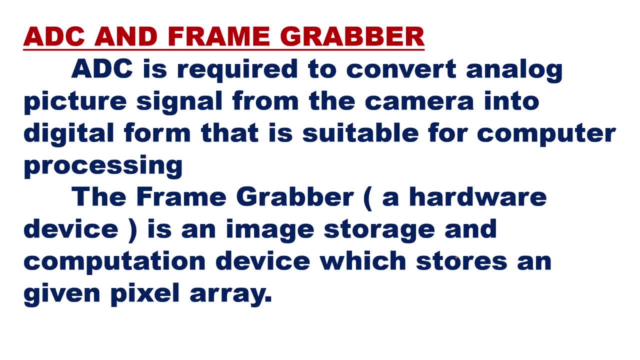 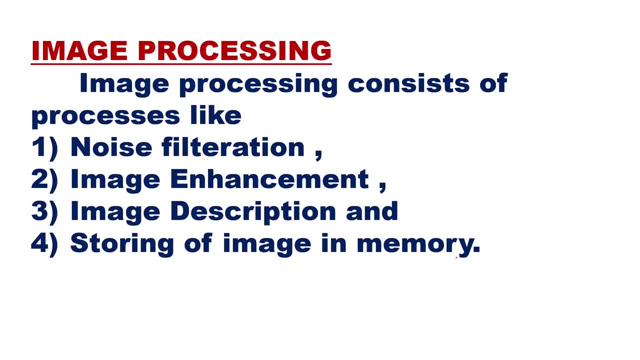 That is, the image is stored in the memory. that is called as frame grabber. Then what do you mean by image processing? That is, when, once the image is stored in the memory, after that the image is taken and it is processed to get the data out of it. okay,